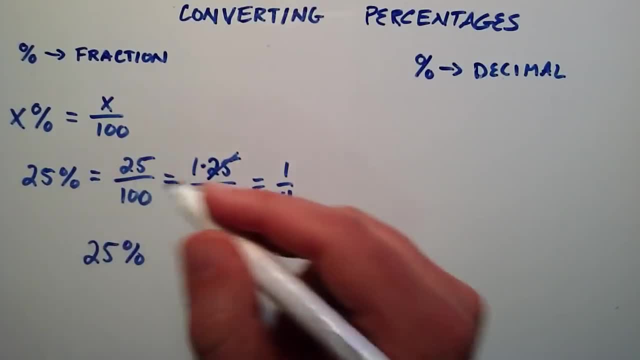 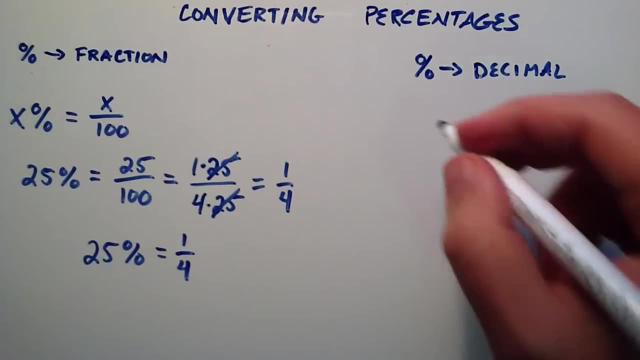 So here we've shown that 25 percent can be rewritten as a fraction and it's equal to the fraction 1. fourth, So how do we convert 25 percent into a decimal? Well, if we write the number 25 here, it doesn't have a decimal point. 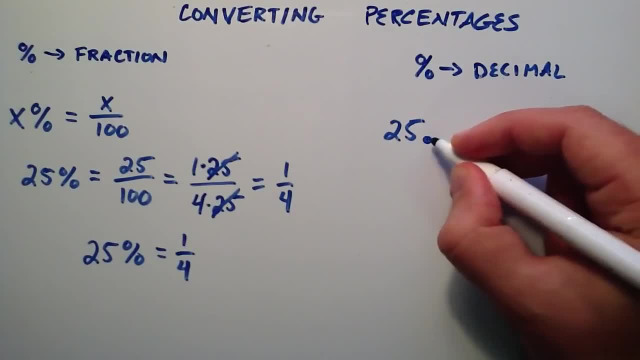 but if we were to put one there, it would go right here. We usually just don't write it, but it's right there. That's where we would put it if we were to. And so we can write 25 as 25 point and then put the percentage sign there. 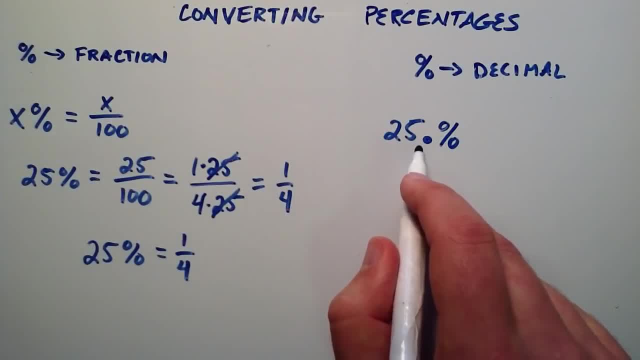 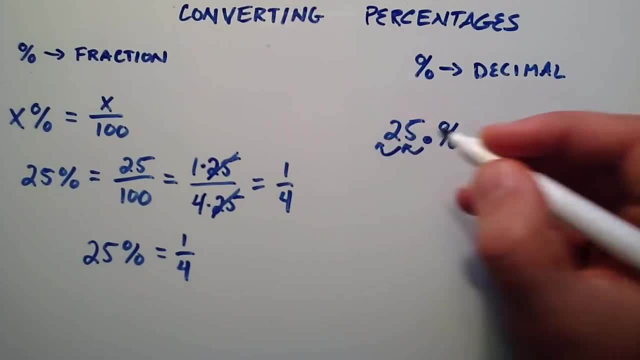 So this is really still 25 percent. So to convert it into a decimal, we simply take that decimal point and move it to u, And then we move the units to the left. So 1, 2 puts it in front of the 2.. 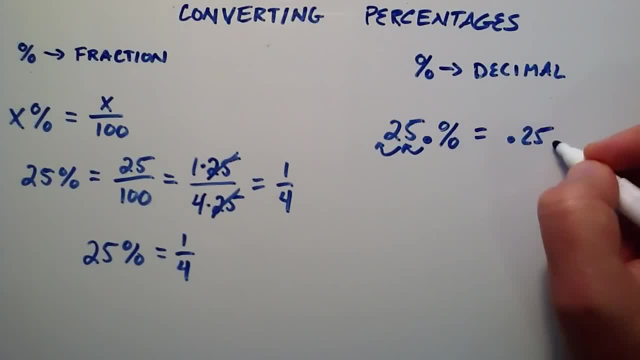 And so we moved it 2 units to the left, and then we get rid of the percent sign, So 25 percent can be rewritten as a decimal 0.25.. And if we were to plug this into our calculator, 1 divided by 4 is equal to 0.25. 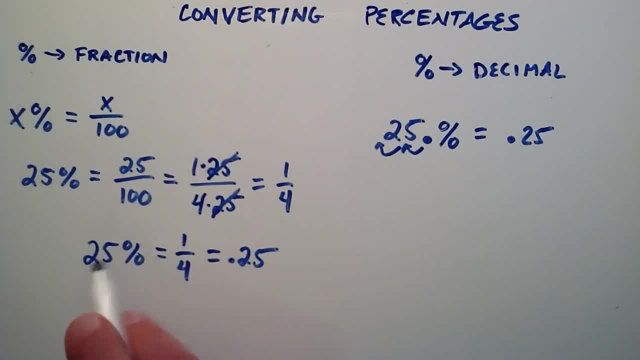 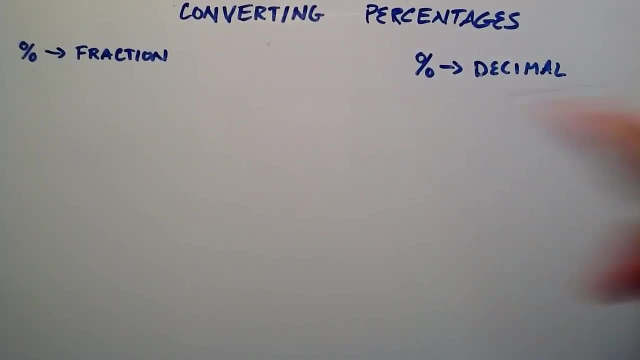 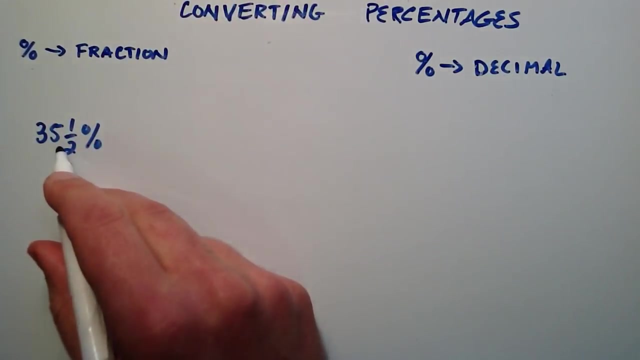 So here's three different ways that you can write the number: 25 percent. Let's do a little bit more challenging example here. Let's say that we have 35 and 1 half percent. Well, the first thing we want to do to convert this to a fraction. 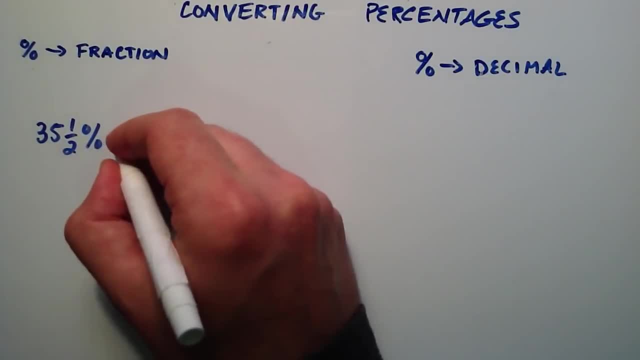 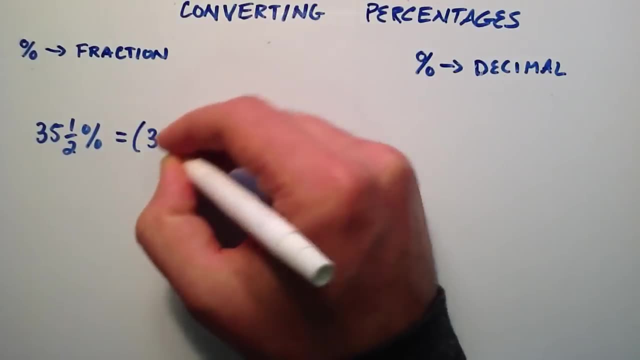 is, we want to put the 35 and 1 half into a different form, So we can rewrite this as 35 plus 1 half, and then the percent of all that. And now what we want to do is we want to put this: 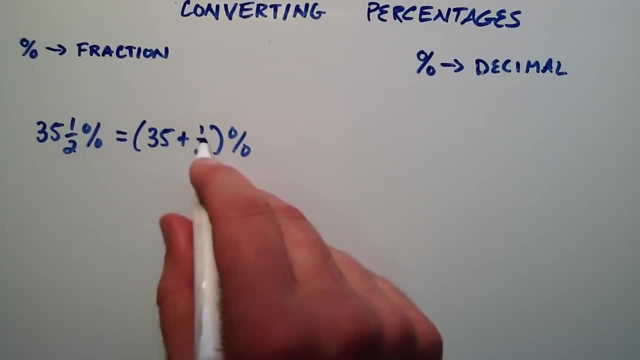 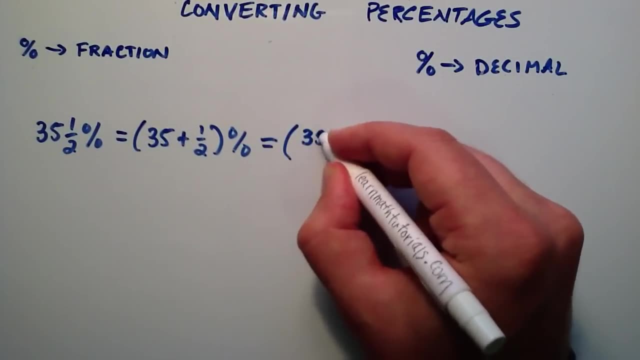 as some number over 2, so that we can add these two together. So we're going to get the same common denominator here, And the way we're going to do that is we're going to multiply the number 35 by the number 1.. 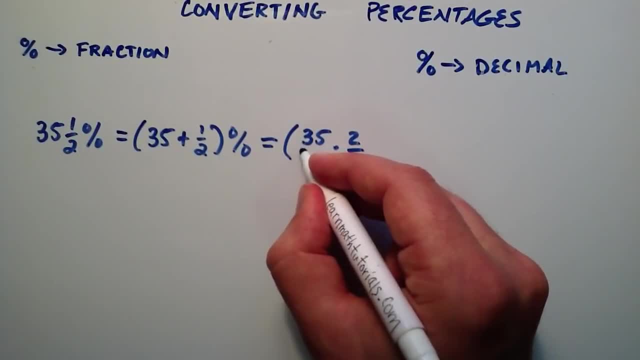 And we're choosing 2 divided by 2.. That equals 1, so we're going to multiply it by that. That's our number 1.. And then we're going to divide it by 1, because that doesn't change anything. 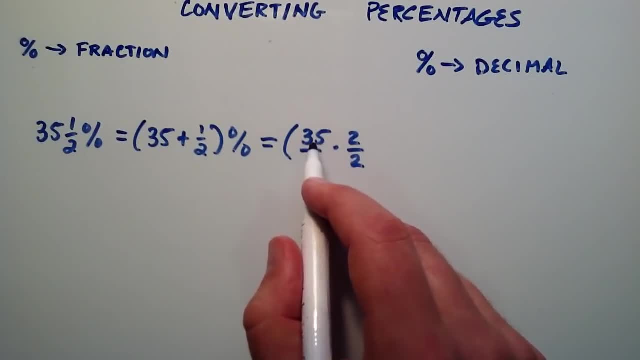 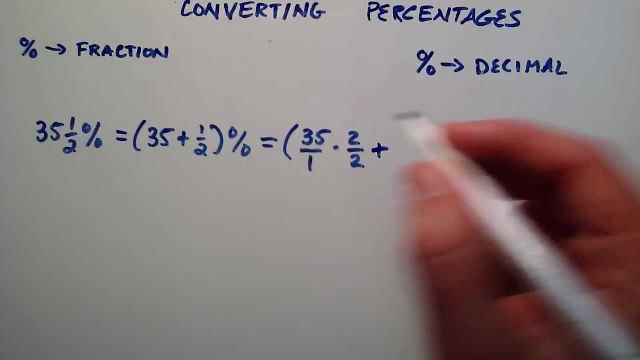 So what I've done here is I'm still left with the number 35.. 35 divided by 1 is still 35. And 35 times 1.. 35 times 1 equals 35. And then we're adding that to the 1 half and taking the percent of all that. 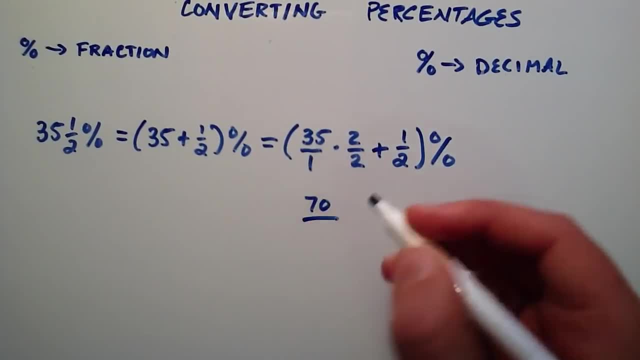 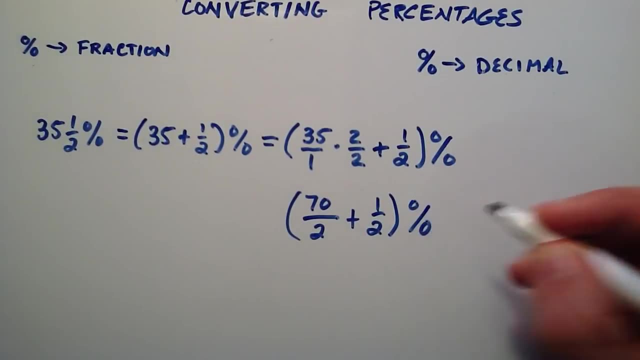 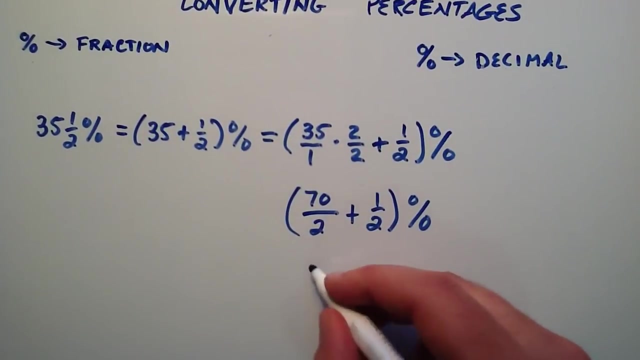 35 times 2 is 70.. 1 times 2 is 2.. And then we're adding our second term, 1 half, putting the percent on the outside, And now we have two fractions with the same common denominator. so we simply add the numerators together. 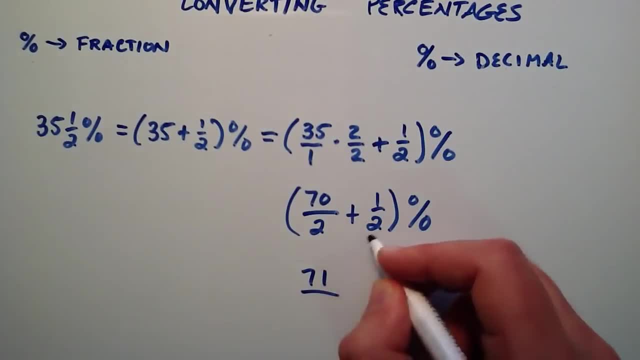 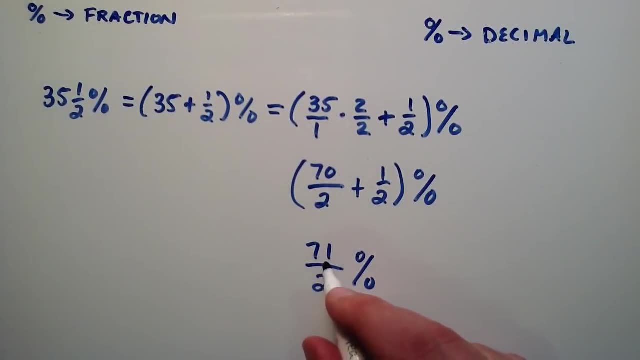 This becomes 70 plus 1, which is 71 over the common denominator of 2 percent. So now this is our x in that form that I had up here. I erased it, but it looked like this: x percent equals x over 100. 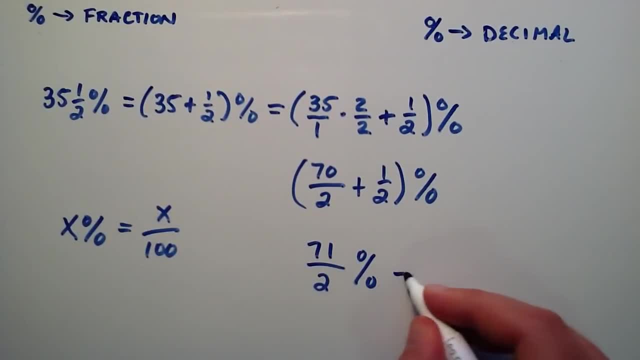 So 71 over 2 is our x. So this can be rewritten as 71 divided by 2 divided by 100. So a fraction divided by 100. And we can actually make the denominator into a fraction here by dividing it by 1.. 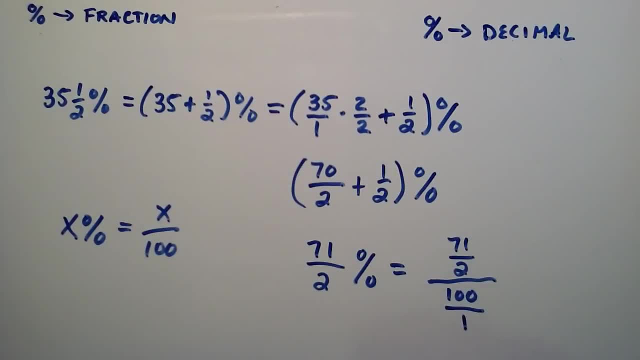 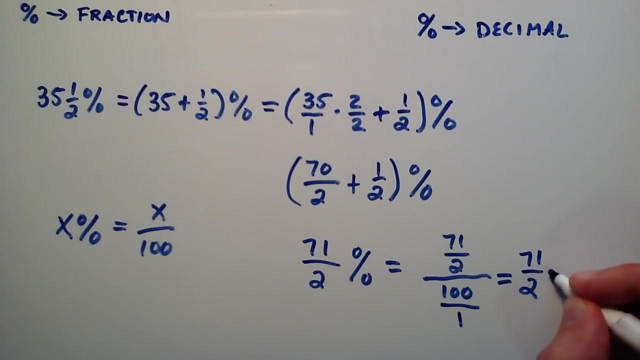 So now we simply have a fraction of fractions And we can solve this problem by rewriting it as a multiplication problem, by inverting this denominator. here We flip the denominator, So we rewrite the numerator here: 71 divided by 2. And instead of dividing it by 100 over 1,. 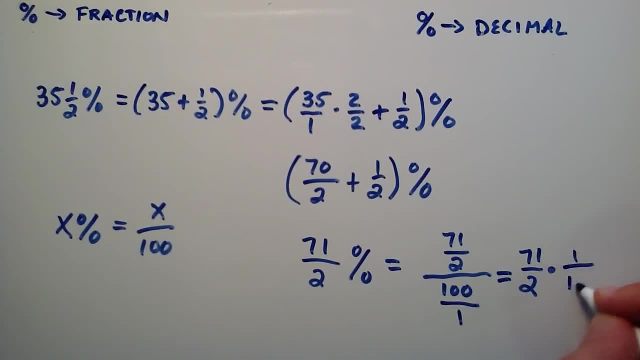 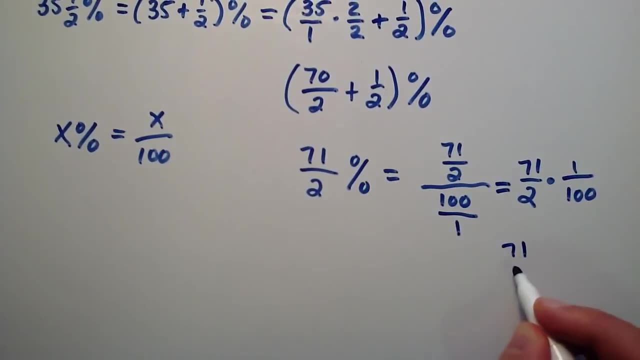 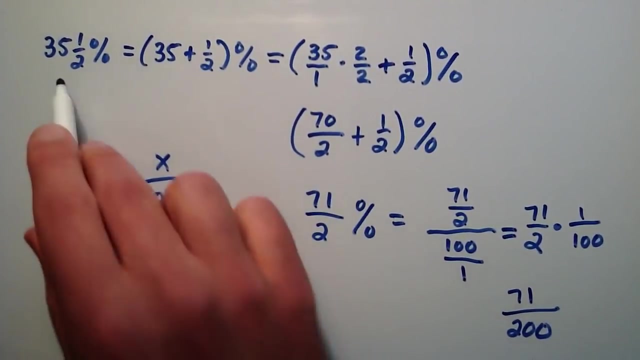 we multiply it by 1 over 100. So now we have: 71 times 1 is equal to 71. And 2 times 100 is equal to 200. So we've converted 35 and 1 half percent into the fraction 71 over 200.. 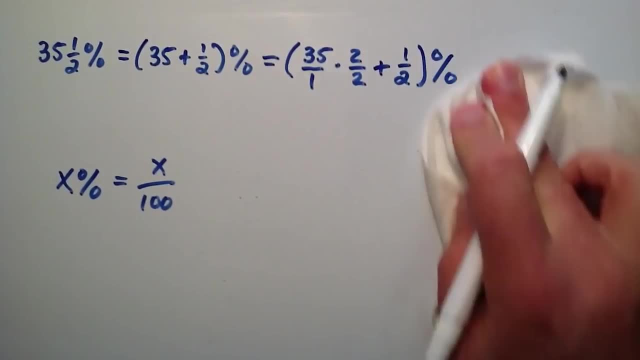 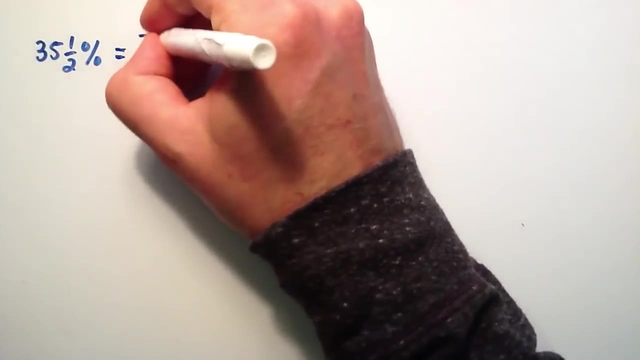 So let me go ahead and just rewrite that next to the 35 and 1 half percent here, 35 and 1 half percent is equal to 71 over 200.. So now what we want to do is we want to rewrite this in decimal form.